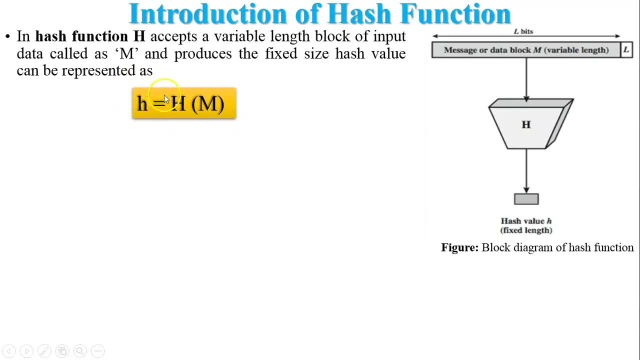 and small h is the hash value. So small h is the fixed length hash value. When hash function provides security, this is called cryptographic hash functions. Hash function protect the integrity of the message. We all know that in code integrity means if message should not be altered by the any other users. 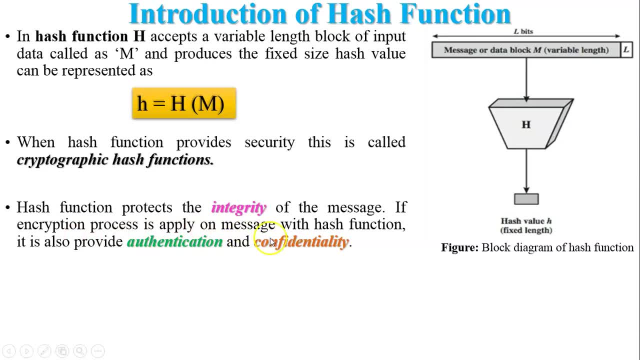 If encryption process is applied on messages with hash function, it is also provide authentication and confidentiality. Whenever we have achieved authentication, integrity and confidentiality so we can say apply the concept of digital signature in the hash function So we can say it is hash code based digital signature. 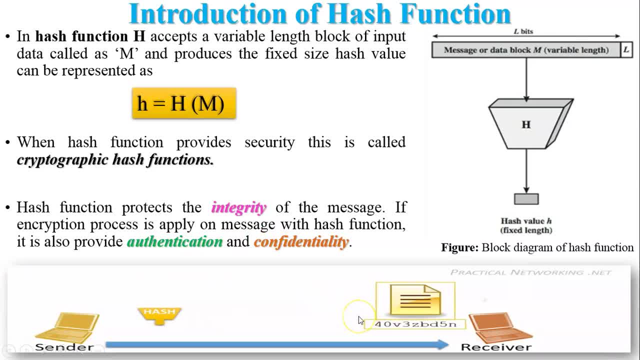 Now this is one diagram To understand the better understanding of the hash function working. So this is one message. Using this message, we have created one hash function. This is hash function value. It is appended to the message reached at receiver side and 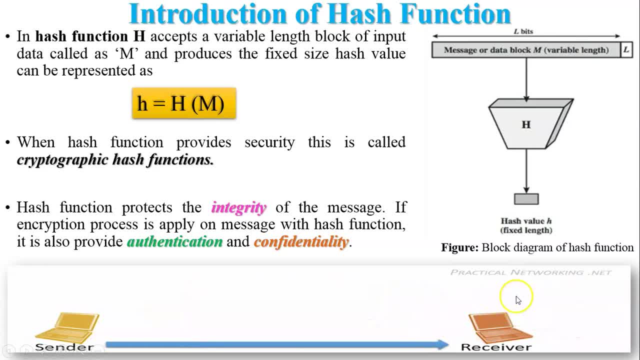 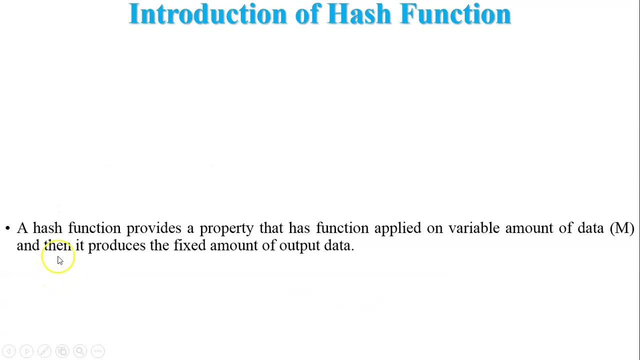 receiver appended value will be removed from the message and store anywhere. And then a new hash value generated from the message and compare both the values. Now check if both values are same, Then receiver accept the message. Otherwise receiver discard that message. Next, a hash function provides a property that has function applied on variable amount. 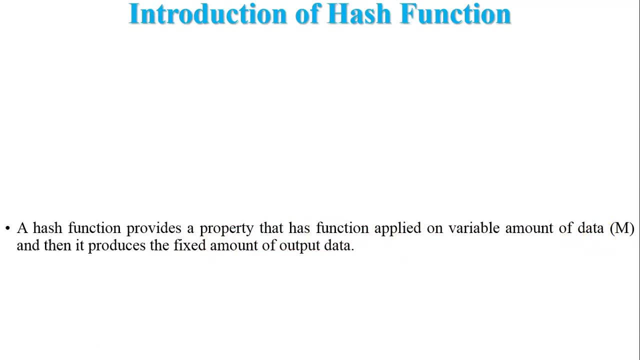 of data m. We have already discussed about that. input of the hash function is variable length and then it produces the fixed amount of output data. We can say it is hash value, small h. Now see one example Here. one message is fox And the hash function created. This is the hash function. 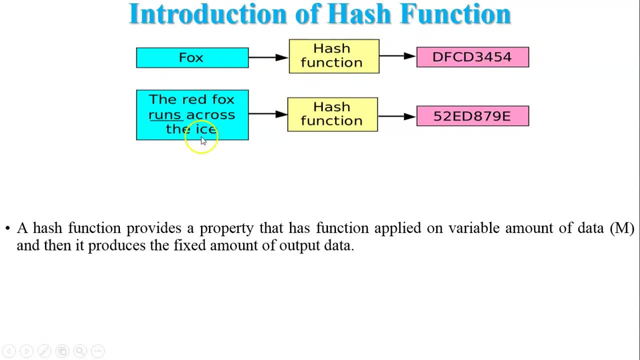 Now another message is: the red fox runs across the ice. This is the another example Now hash function created of this function is this: So hash value of both the message are same, But the length of both the message are variable. So this is one of the property of hash function. 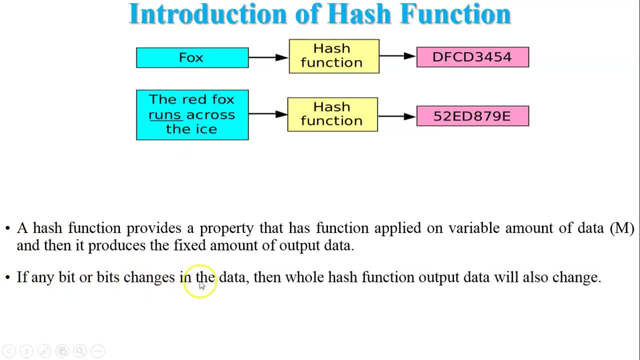 Next one: If any bits or bit changes in the data, the whole hash function output data will also change. It means if I have changed any of the word or any of the single bit So it produce different hash function. Now see another example. 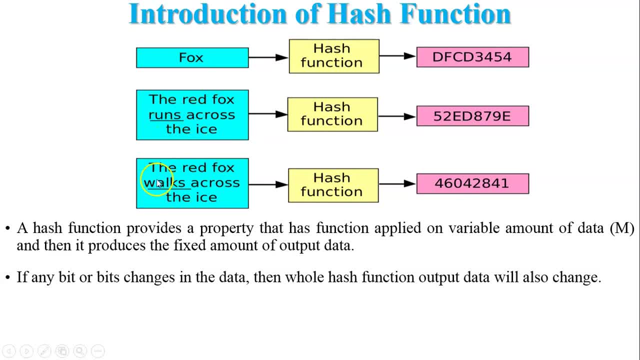 One is that the red fox runs across the ice and second one is the red fox walks across the ice. Now generate hash function of both the input message and both are different Now you can see over here. So this is the another property of the hash function. 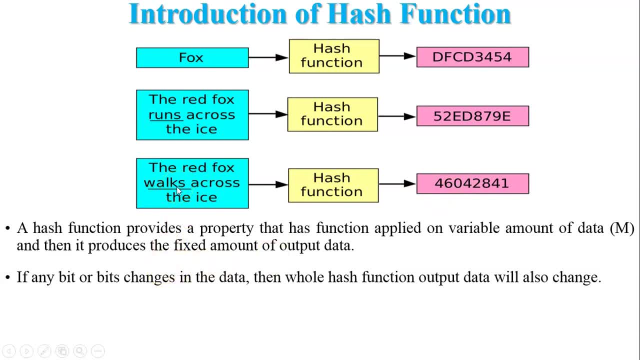 So if there is any change in the bits or Or any bit, whole hash function output data will also change, So hash value will be changed. Next, cryptographic hash function is one way function which is practically infeasible to invert. It means this is the message fox: now generate new hash value from the hash function. 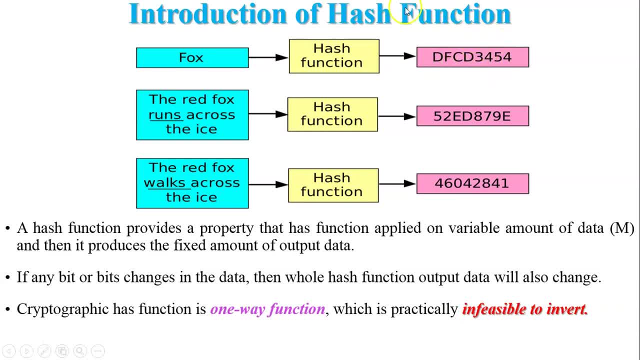 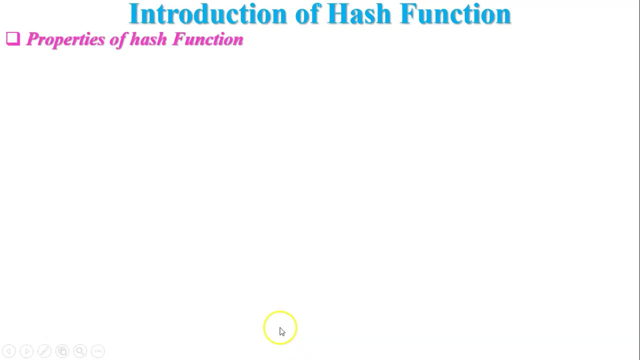 Now, if I have this hash value, I cannot get the original message from the hash value, So this is called one way function So, which is practically infeasible to invert. The most popular hashing algorithm is MD5 and SHA. MD5 is message digest 5 and SHA is secure hash algorithm. 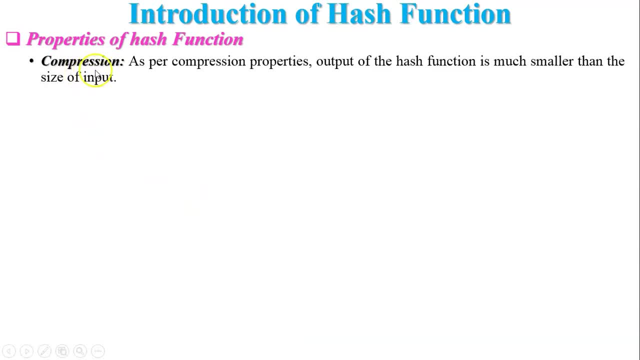 Now properties of hash function. First property: compression. We have already discussed about that. there is variable length of input is given but fixed value of the hash, fixed size hash value will be produced. So compression, as per the compression property, output of hash function is much smaller than. 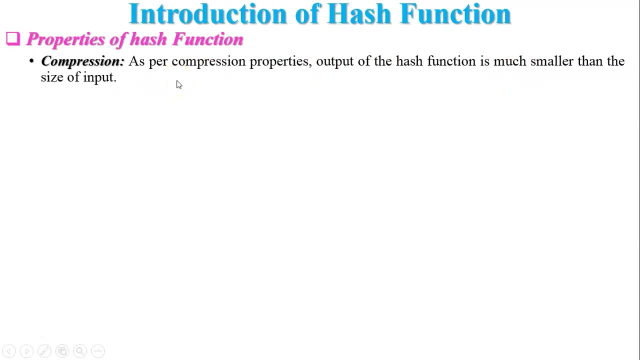 the size of input. If size is 1024 bit, if you are using SHA 1, there is 160 bit hash value is generated. Next one preimage resistance. Preimage resistance means difficult to find the input from the given hash function output. 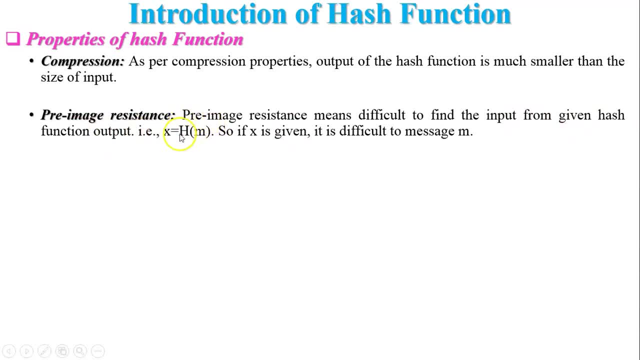 If there is one message, The hash function of this message is applied and generated. hash value is X. So if X is given, it is difficult to message M. So this is called preimage resistance or we can say it is one way property. Now, third one, weak: collision resistance. 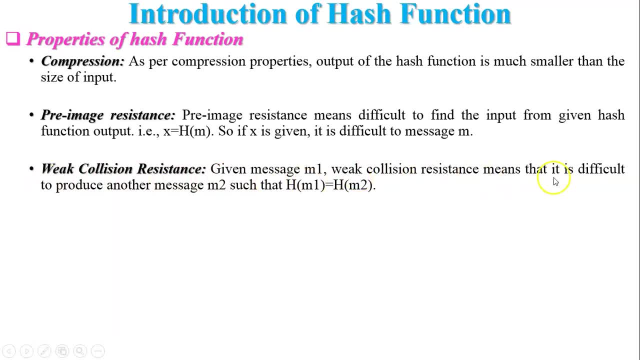 If given message M1 in weak collision resistance means that it is difficult to produce another message M2, such that H of M1 is equal to H of M2. So we can say, Ah, If given message M1 and M2. So we cannot. same hash function will be generated using the different messages. 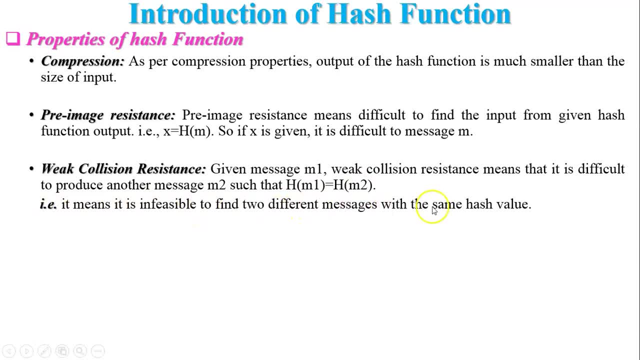 So it means it is infeasible to find two different messages with the same hash value. Fourth one: strong collision resistance. there is some difference in weak collision and strong collision. We will discuss later on. strong collision resistance means that it is difficult to find any two. 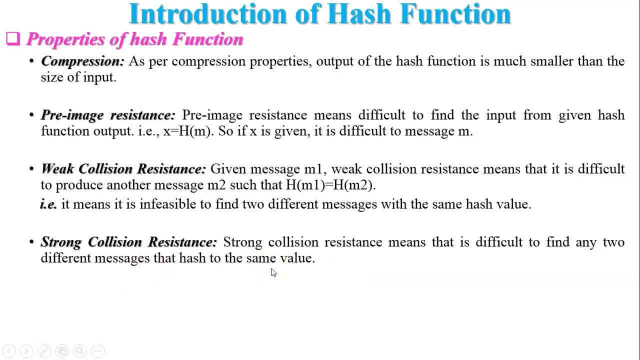 different message that hash value to the same value It means It is. It is difficult to find M1 and M2 such that same value: H of M1 and is equal to H of M2.. So here everybody think that weak collision and strong collision resistance are the same. 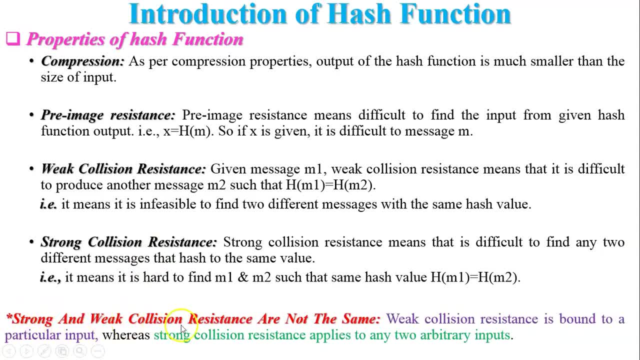 There is small difference between them. Now, strong and weak collision resistance are not the same. Weak collision resistance is bound to a particular input, whereas the strong collision resistance applied to any two arbitrary inputs. So there is the small difference between strong and weak collision resistance. 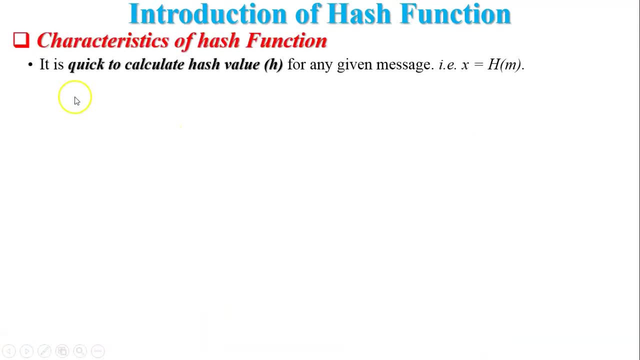 Next characteristics of hash function. first one: it is quick to calculate hash value h for any given message. it means x is equal to h of m. now m is the message, hash function is processed and hash value is generated: x. second one: hash function h can be applied to the variable length of 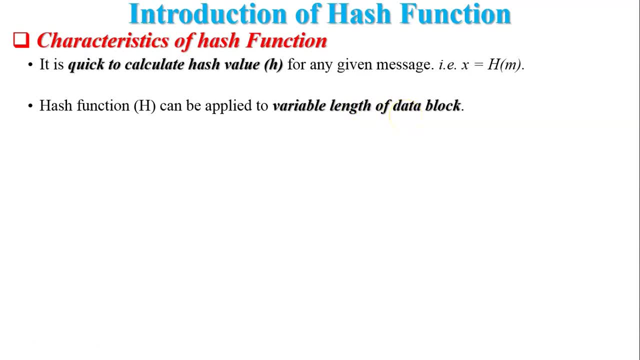 data block. we have already discussed this is the one of the good characteristics of the hash function. there is a small change in a message should change the hash value. so this properties is mostly used for the check the integrity or verify the integrity of the message at receiver. 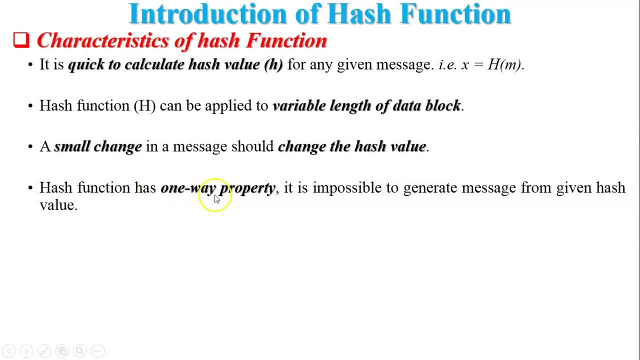 side. fourth one: hash function has one-way property. it is impossible to generate message from given hash value. it means if any attacker get the hash function of that message, so attacker cannot decrypt or cannot get the original message from that hash value. fifth one: the hash function uses all the input of the data. if all the 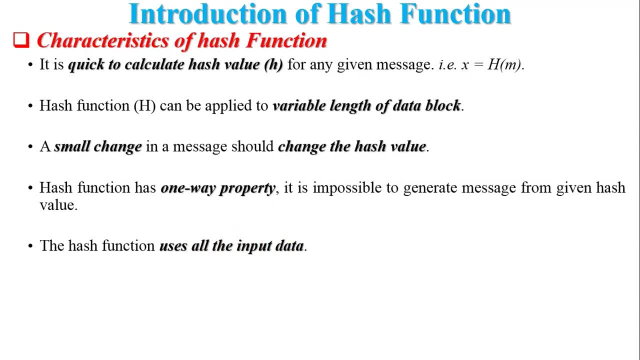 input of the data is not used in the hash function, so it may be generate the same hash function, so we can say it is. it may be generate a weak collision or strong collision resistance. next one: the hash function uniformly distributes the data across the entire set of possible. 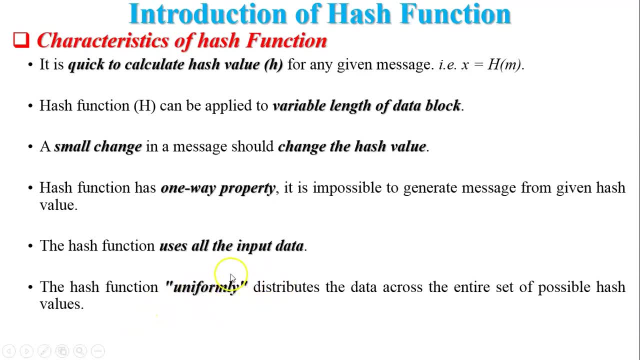 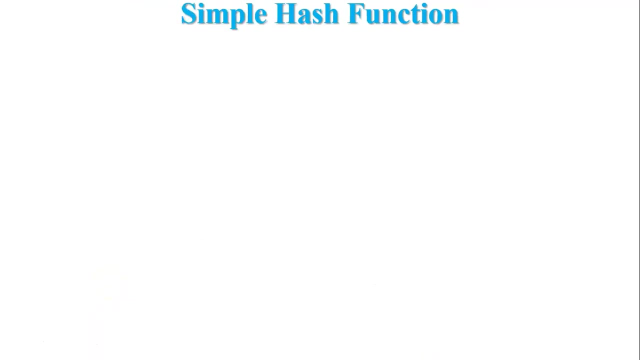 hash values why it is uniformly distributed. if it is not uniformly distributed, then it distributes. it may be happen weak collision or it may be happen strong collision, resistance. and the last one, the hash function, generates very different hash value for the similar message. if both the message are same, hash value should be different. now, simple hash function here, there. 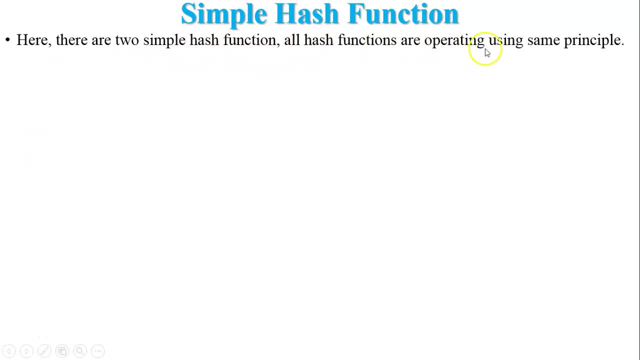 are two simple hash functions. all hash functions are operating using the same principle. now discuss about first one. first, the message file is like a simple input. it open a sequence on n bit blocks. it means if your message file is too long, so it is converted into n bit blocks. now, second point of 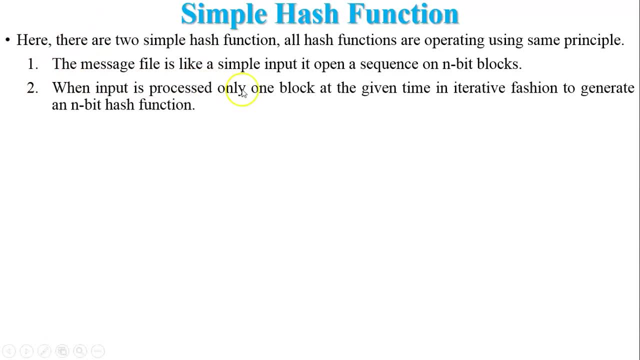 the first hash function. when input is processed, only one block at the given time in iterative fashion to generate an n bit hash function. now see one example. the simple hash function is the bit by bit x oring done of every block. now see, this can be shown. shows the following ways. first one, the 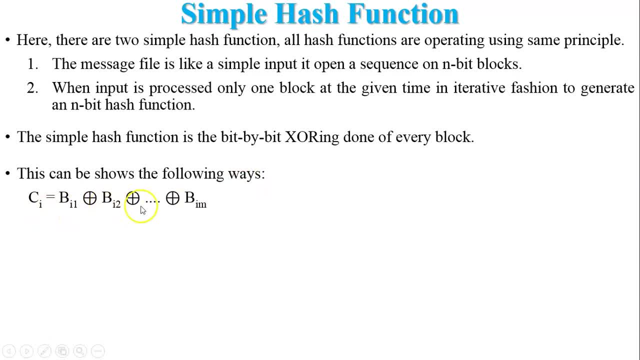 equation ci is equal to bi 1 x or bi 2 x, or up to x, or with bi m. now check this table. this is the block by block x oring. so here i can see first one. ci is the ci is ith bit of hash function code now. 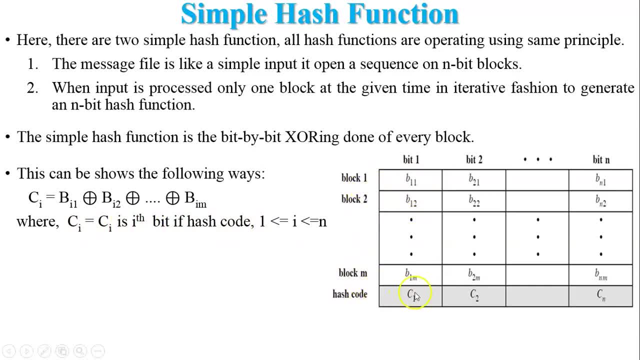 check. this is block 1, block 2 and this is block m. now all the blocks. first bit is x, ored with each other, and it generates c1, or we can say this is ci, because it is in general form. next, what is m? m is the blocks. how many blocks are created? 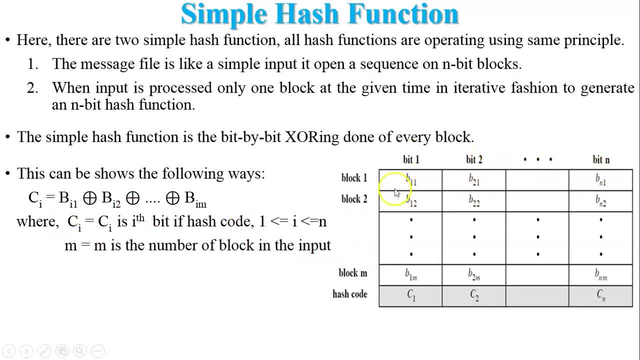 and n is the bit of blocks for one block. so m is the number of blocks in the input. bij is equal to ith bit in jth block. now check over here, block 1, bit 1. so this is b 1: 1. so i can see, or i can say first bit of the first block. now this is the